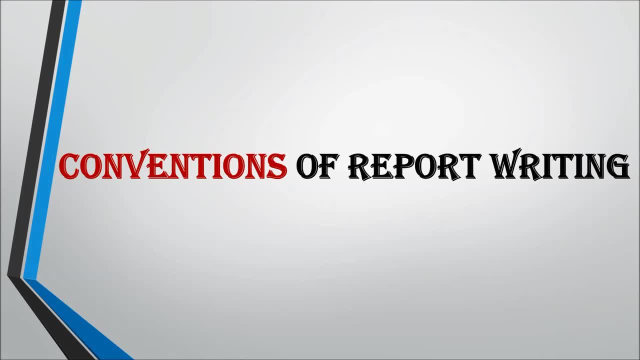 conventions. what does it mean? It basically means a prescribed method, a prescribed way that is universally acceptable. So we are going to learn about that art of writing report on the basis of field work which is conventionally accepted universally. So the entire world accepts a particular convention, For example, drawing of a map in geography. we all know that conventional symbols, their importance, the importance of 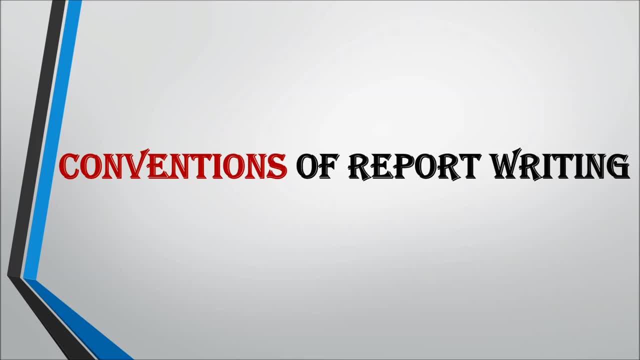 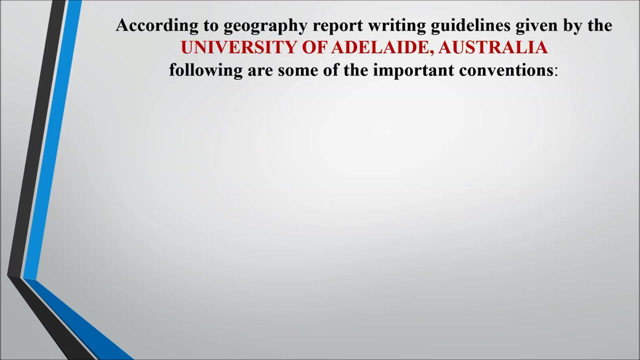 directions. So, similarly, we have certain conventions in report writing as well. So please focus upon those conventions and understand that these conventions are necessary in order to write your report in a comprehensive and excellent manner. So these conventions have to be kept in mind while finally drafting your report. So what are the conventions? According to the geography report writing guidelines given by University of Adelaide, Australia, we are having certain 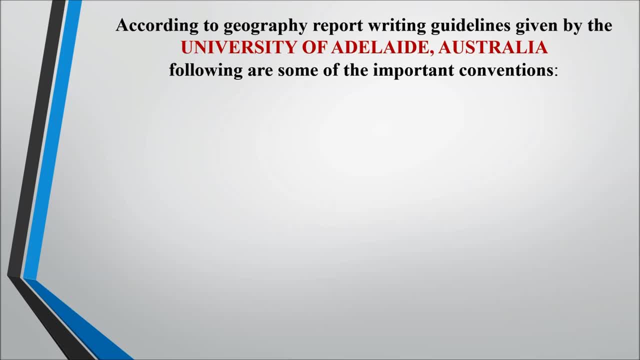 we can see is universally acceptable. so let us see: first is the name of organizations. so whenever we say a particular organization, for example, national atlas thematic mapping organization, so whenever we are writing any organization, so first we need to write the full name of the organization and then in bracket we need to write the acronym. so never just write the acronym or 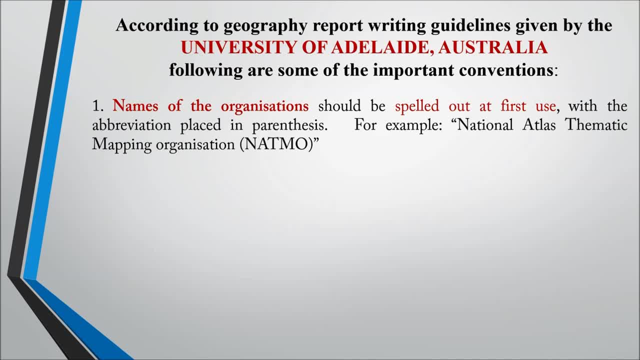 just leave it like that, or maybe you can do the reverse. many a time people do it, so remember: any organization has to be written in this format, as you can see here: national atlas thematic mapping. organization in bracket, natmo. so this is the way you need to write. 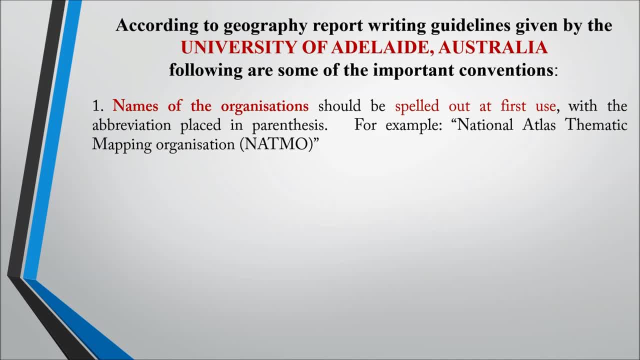 the name of any particular organization. that is part of the reference. so that is one of the conventions. let's look at the other. researchers must not use apostrophe. remember that an apostrophe is not needed when we are writing dates in numerical representation, for example, 1950s. can you see? 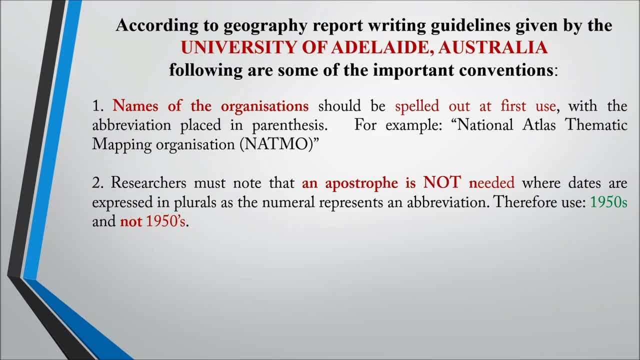 here on the screen. so simple: 1950s is 1950 and s. apostrophe is not needed. that's not a proper convention. so if you are using apostrophe, it's not a convention. remember, whenever you're writing a date, just write the date or the year and just add s to it. don't use apostrophe, alright. 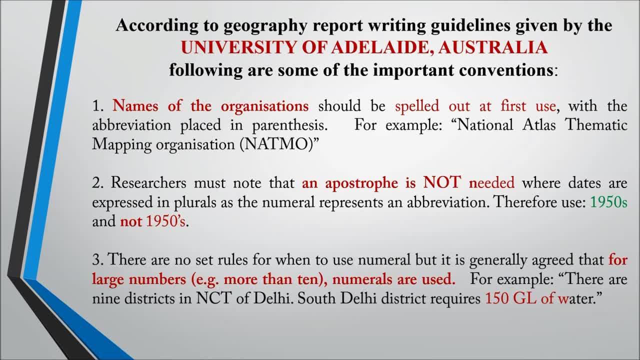 now, the third important convention is that there are no set rules when to use numeral, but generally the general convention, the general agreement, is that if the numbers are large, it means if it is 0 to 9, then it's fine, just use a single numeral. but if the numbers are large, then proper numerals. 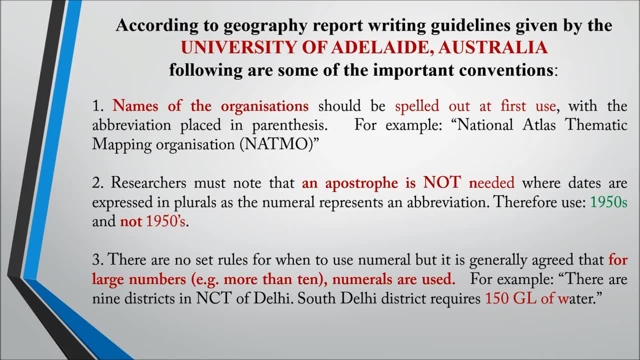 are used. so if 0 to 9 is there, then you can write it in alphabets, for example o-n-e-t-w-o-n-i-n-e, but if it is 150 gallons of water, so 150 as a numerical, as a number, you can write when it is more than 10. 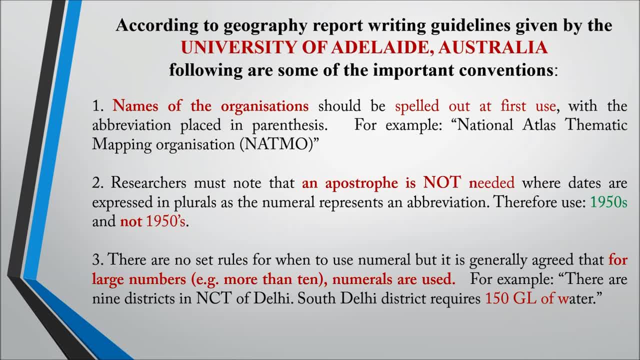 so that is a basic, acceptable convention for report writing. so remember, whenever you are using the terminologies as numerals, okay, it should be at least more than 10, because 0 to 10 value you can write in alphabets. all right, now let's look at the other convention. so for calendar years, it's. 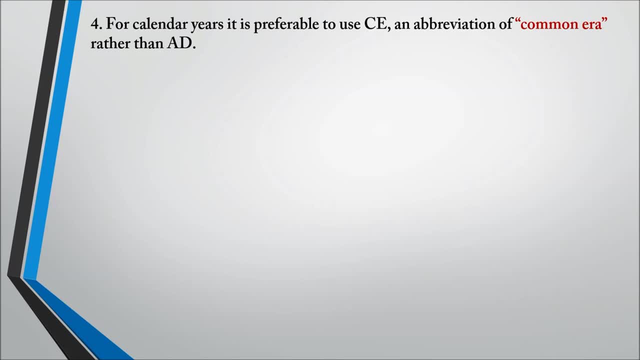 era ce, because the world uses common era. now. ad is out of fashion, so ad is not acceptable. now. common era is ce, so for year write ce, right then. fifth one, the international system of measurements. that is we already know. si units should be commonly used in report. always use a standard international. 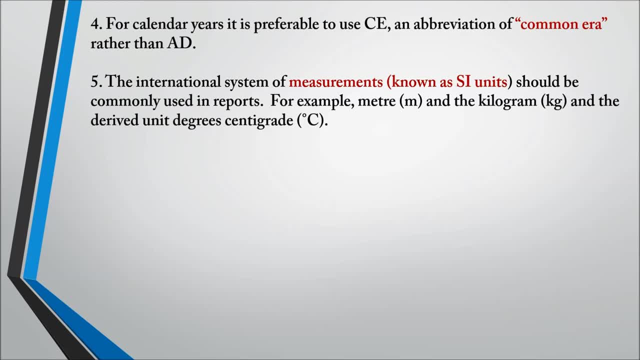 system of units. for example, meter is m, kilogram is kg, centigrade is degree c. so remember, always use standard units. okay, now numerals and units of measurements should require a space between them. for example, do not just write one and without giving space right: km. so one space, km thousand. 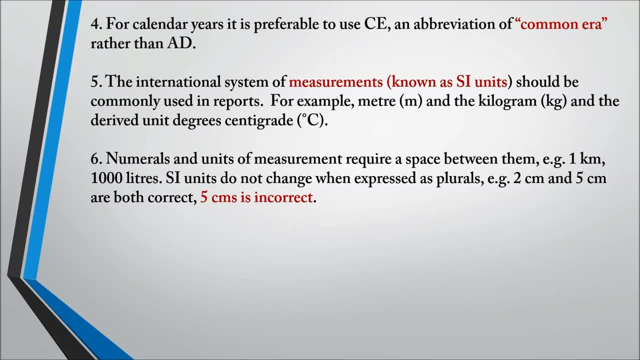 space liters, so remember, and whenever you are using plural in that. so don't write two cms, five cms, five cms or two cms is wrong. remember the unit would be cm itself. unit would be km itself. you don't need to add s to the unit. this is a common mistake. everybody does whenever it's larger. 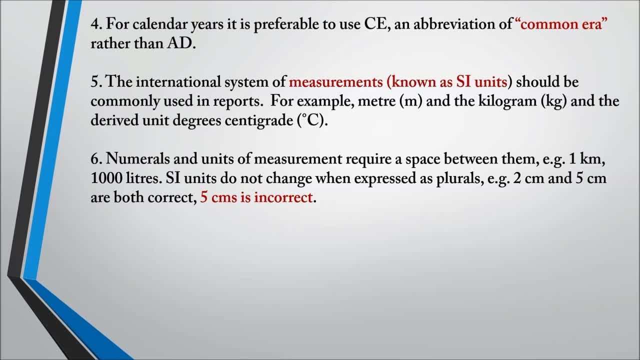 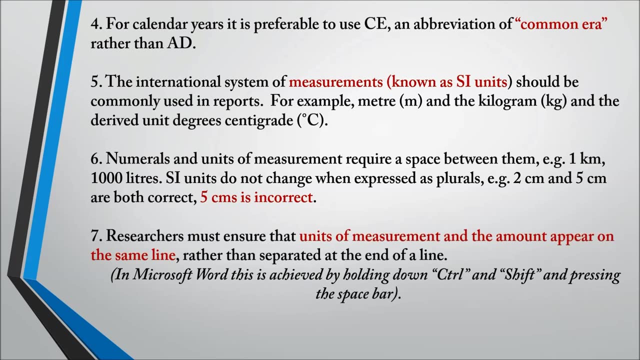 amount many times in plural. people try to express in kms, cms, so this is not correct. okay, just write km or cm. okay, but space must be there between the number and the word. okay, now researchers must ensure the units of measurement and the amount appear on the same line rather than separated at. 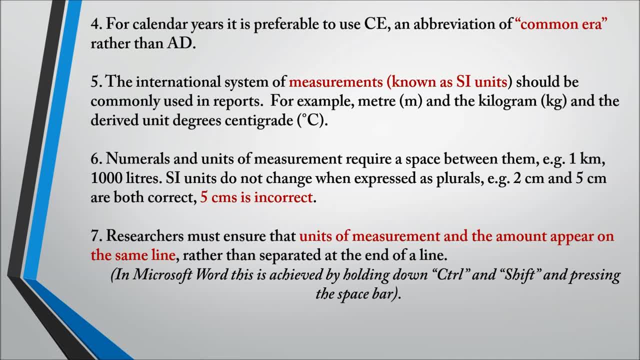 the end of a line. so wherever you are using a particular number, you should write the number in a particular unit of measurement along with that number. it you should not change the line. okay, always remember you should fix it in the same line. for example, in many tables people tend to write: 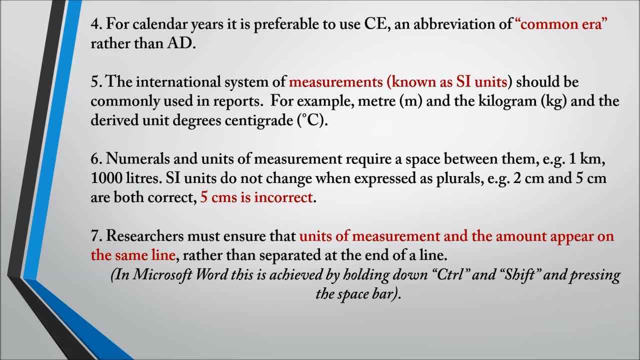 units of measurement below the numbers. so no, always write that number and adjust as you using the control shift, okay, and space so you can adjust your number. and in bracket, if you want to write unit of measurement, so please make it in the same line. that is a convention of writing. 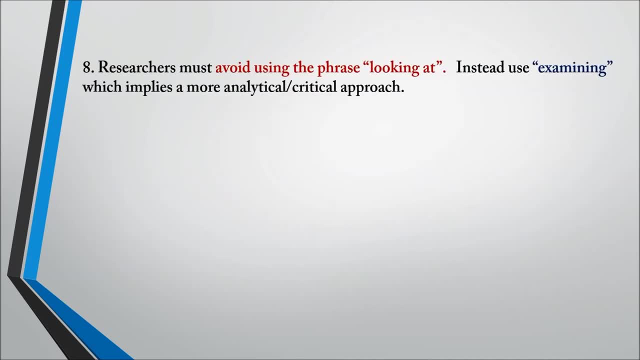 all right now. researchers must avoid using phrase such as looking at, so this is not the way we speak. has to come into the narrative. always remember: whatever you are writing is formally structured. so instead of looking at or seeing okay, or visual or any such statement, write examining, so examining. 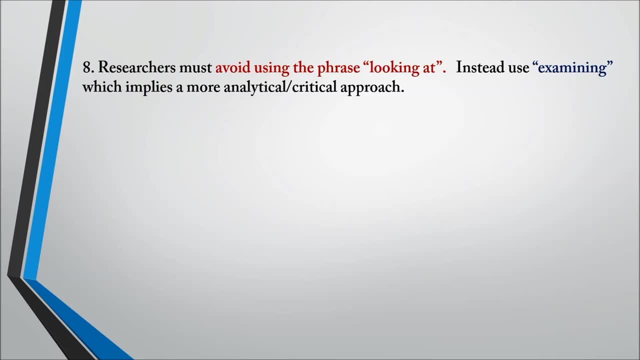 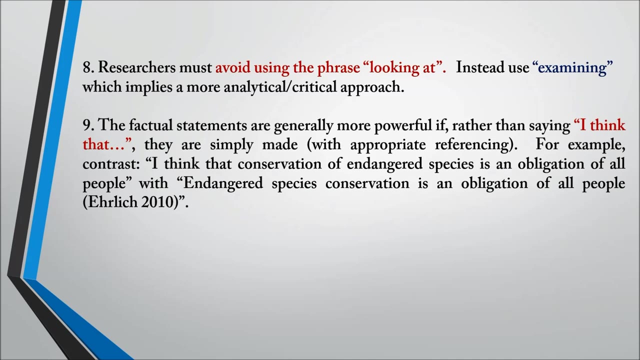 is talking it making it more sensitive. it's saying it is more critical, analytical and scientific in the narrative rather than just simply looking at all right, so don't use this phrase whenever possible. okay, the factual statements are generally more powerful if you don't use a phrase, I think. 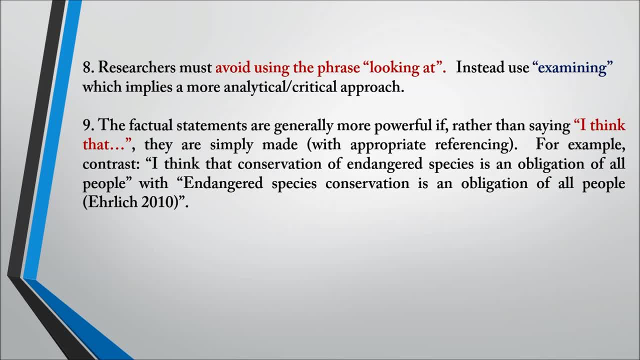 that always write the statement and, in bracket, quote the author. don't write I think, or she thinks, or he thinks. no, that's not a proper way. so always use appropriate referencing for a particular statement of knowledge, like shown in the example. so endangered species conservation is an obligation of all people. bracket erich 2010. right, so don't use. i think that. 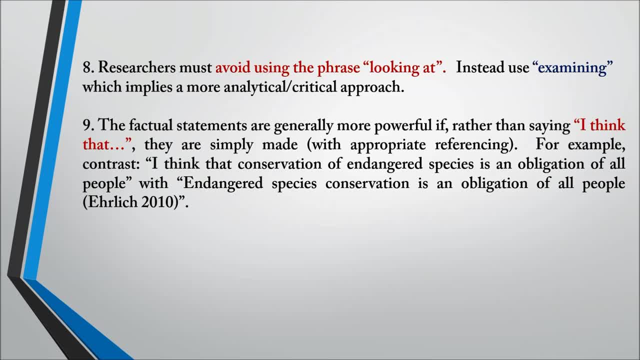 okay now. researcher must avoid overuse of the term issues. this is very common problem that i find in all the students and researchers that they always tend to speak lots of rather than problem and challenges in the study area. they talk lots of issues. so what happens? issue is a negative word. 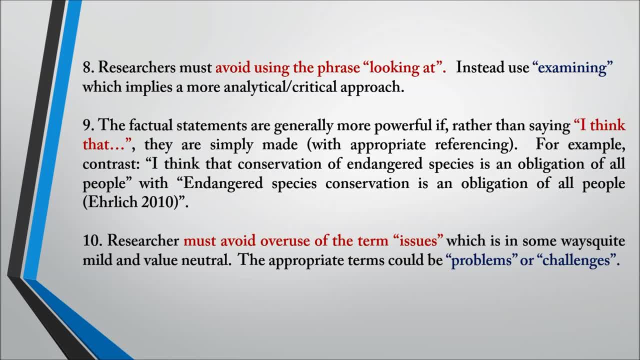 remember, don't make lots of issues by writing too many issues in your terms, okay, so avoid over usage of the term issues. rather than write about problems, challenges, okay, these are the substitute words. don't use issues everywhere. okay, now, avoid the use of terms that are gender biased, for. 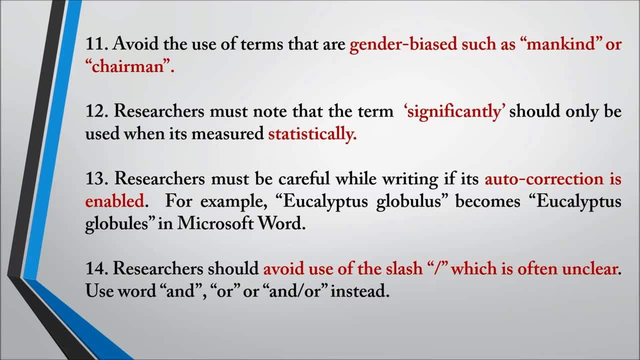 example, mankind, okay, it's not mankind now, it's humankind, okay, chairman. so wherever you find this gender biased term, find an alternative. try not to use a gender bias term. all right, researchers must note that term significantly should only be used when it is statistical analysis going on. many a times we interchangeably use the word important and 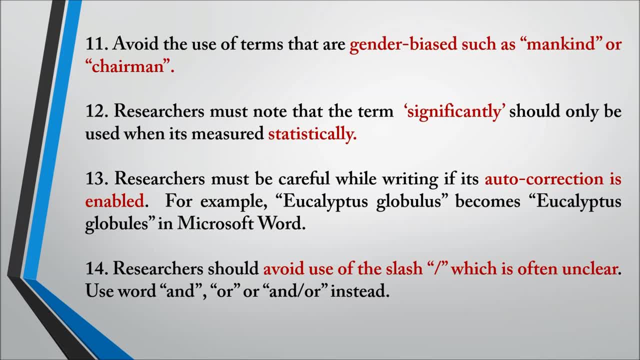 significant wherever we want. but you know what is the significant difference, main difference between these two? significance is statistical, but importance is general. so if you are not giving any statement that is statistically giving any data, then don't use it significantly. so write importance in place of significance. significance level. significance is only 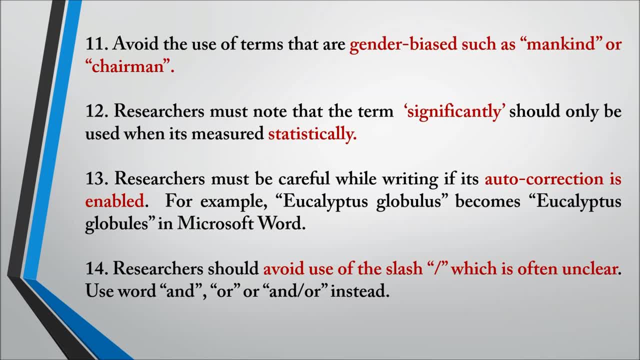 when we are stating something statistically. otherwise use the word importance unless you are using something statistically. okay. now if your auto correction is on, it may create trouble. so always remember auto correction is also handy at times but also can lead to many trouble. for example, if you see here, eucalyptus globulus becomes eucalyptus globules in microsoft几cento. you see eucalyptus becomes eucalyptus globules in microsoft terms. so, for example, eucalyptus in Microsoft terms is the most important or important thing in the weapon in the world. 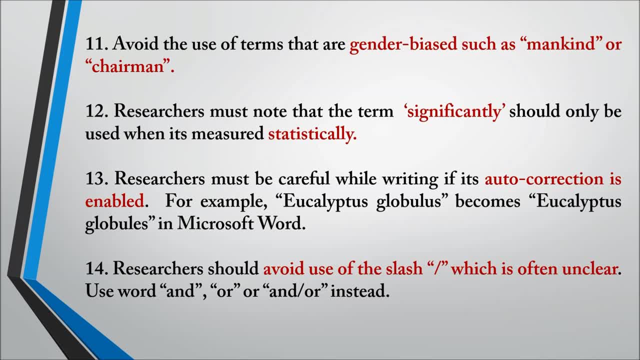 adjus bc. adjus, bc in Microsoft Word, so auto correction can cause lots of problems, so be aware of it. and 14th point: if you see, researchers should avoid use of slash. okay, because many times we want to use the word and or, but we tend to forget that and just. 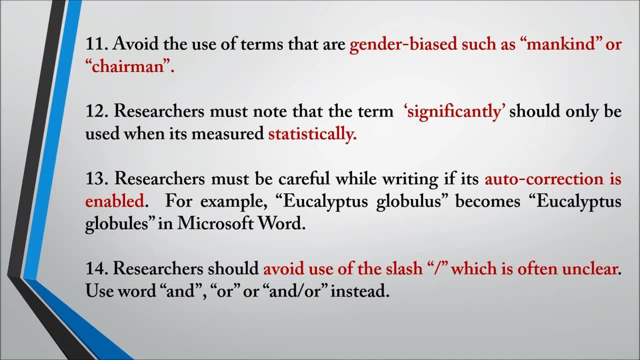 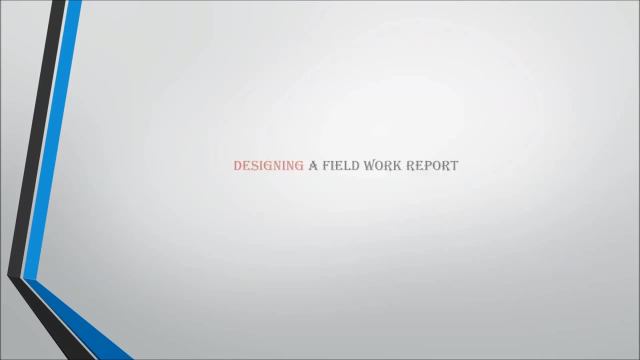 put a slash. so avoid the usage of slash rather than use. and for the separation, or or for the separation, don't use the word or the symbol slash. all right, so these are largely the symbology and all the conventions of report writing which we discussed today. so these are very fine points while designing a field work. 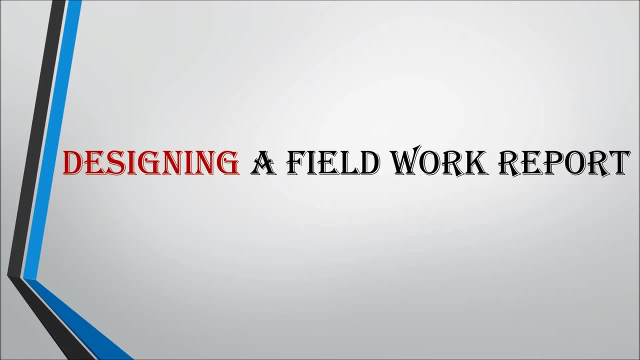 you should remember all these conventions that we talked about. how many conventions? basic, basic, little little things- 14 conventions. so whenever we are writing our report, we should avoid making those mistakes which are important and we should avoid making those mistakes which are important and not part of the fieldwork writing okay. so please avoid all those parts that are. 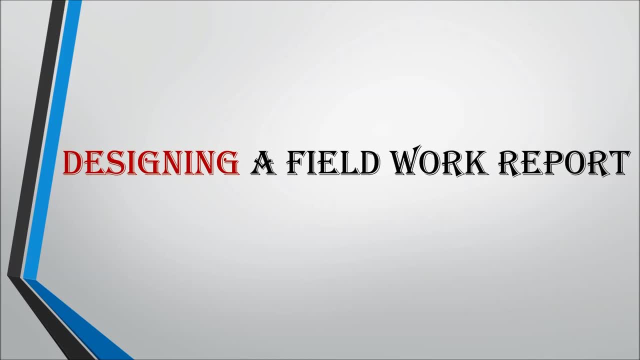 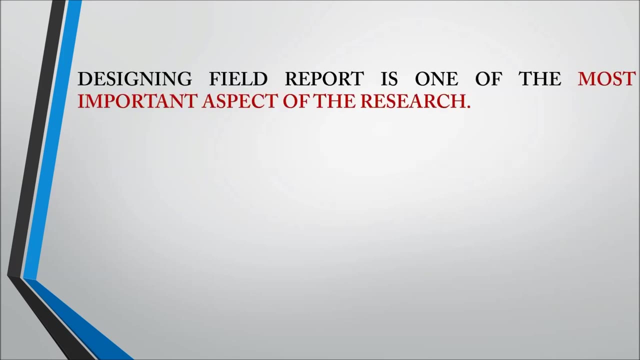 not the part of convention. so follow the conventions. now let's talk about designing a fieldwork. when we're talking about design, it makes sense that how we are going to proceed in the arrangement of final report. so let's look at that. designing field report is one of the most important aspect, because this is 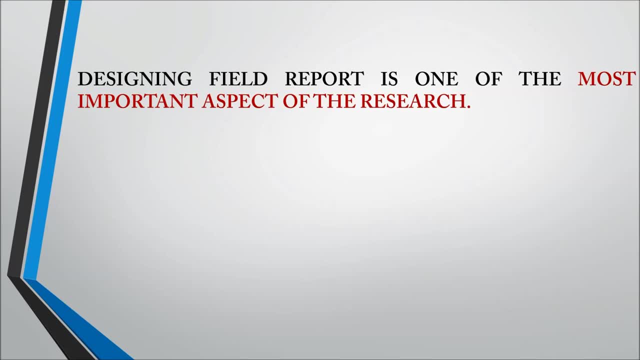 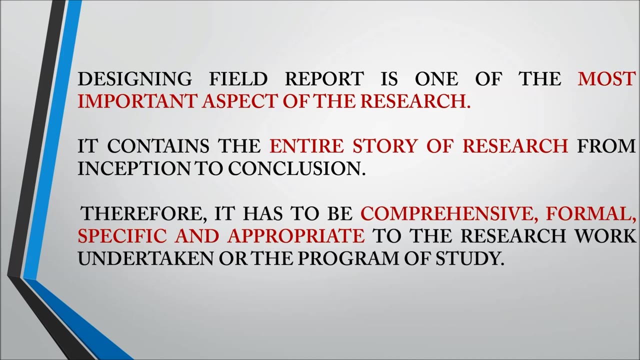 what your entire result is right, so design has to be very much important now. it contains entire story of your research, right from inception to conclusion, so it becomes one of the most important point, isn't it? then it has comprehensive, formal and specific and appropriate. you know it should be comprehensive, that we already 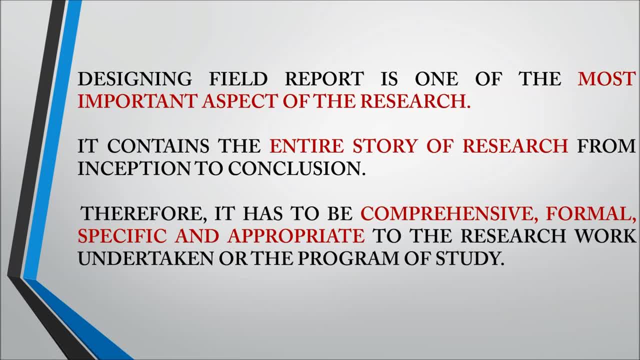 have been talking about it in all the sessions: formally structured, very to the point, very appropriate usage of data and method, and everything has to be stated clearly. so it has to have a proper, fine design, isn't it? so a standard field report consists of six chapters. I am 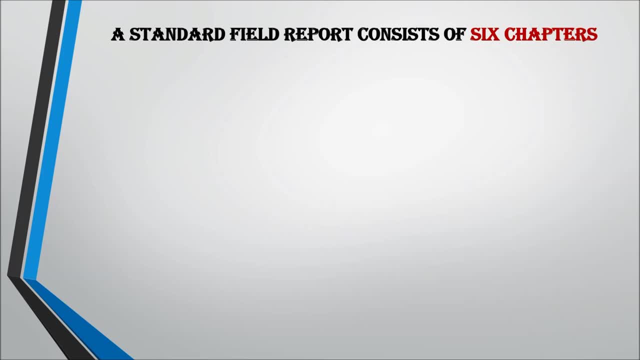 talking only a standard report can also vary. some reports may have only five chapters or four chapters, some may have seven to eight chapters. so, but a standard, what I am giving you is six chapters. all right now see, first chapter is introduction. so what does it include? it's basically includes the research problems: review of literature, objectives, research methodology. 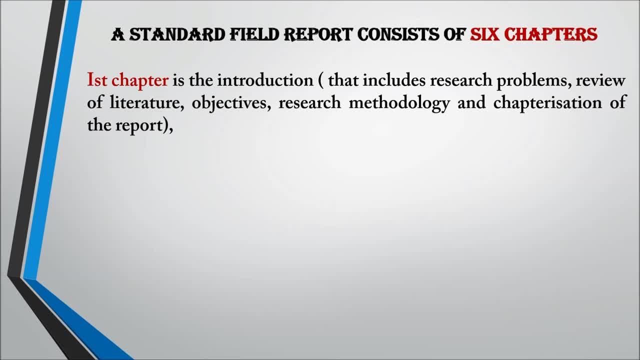 and the chapterization of the report. so first chapter is basically talking about the entire synopsis of your work. okay, the prelude of your work, that. what have you presented further in the entire report, isn't it? so if somebody reads your first chapter, he would understand that. what is coming in the second, third, fourth, fifth chapter, what is finally done in this? 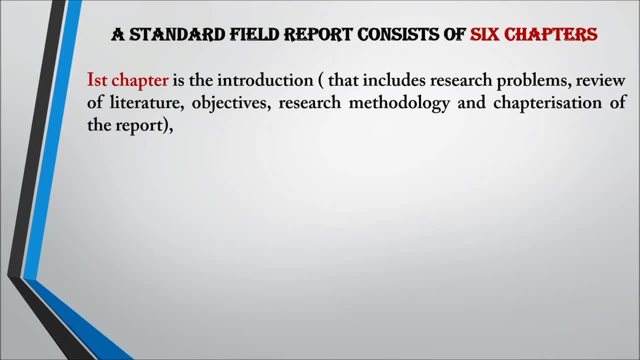 research. that's why it is the introduction to the research. so always remember, make it comprehensive introduction with all these research problems, questions, review of literature, objectives, research methodology and so on, and so forth, and so forth, and so forth. and research methodology and ndtet, or the final chapter, ization, you're doing it, finally all. 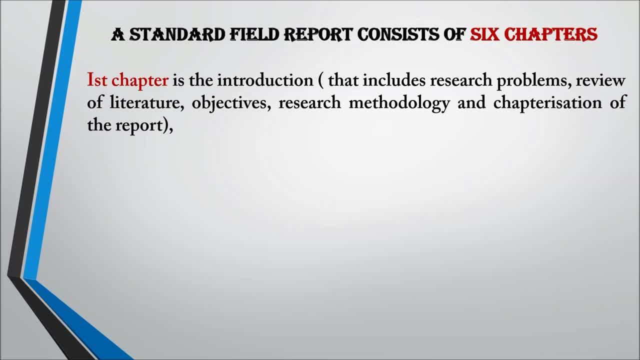 right, but in synopsis stage just like a tentative chapter ization. so synopsis, when we do it for a plan B, Best, then it is required right now. second chapter is essentially geographical profile of glossary Because we are talking about a particular field, so it has to have. 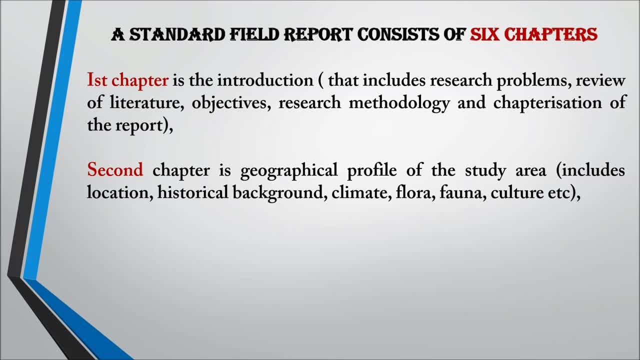 the importance that it deserves, isn't it? so what is going to be the part of it? location, a historical background, ​​climate, flora, fauna, culture, and you can increase the list. okay, so it has to have the entire as much as possible as part of the geographical profile of study area in the second chapter. right then? third, 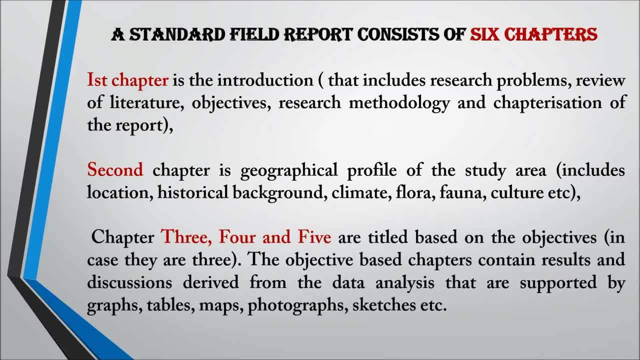 fourth and fifth chapter are going to be entirely based on the objectives that you have selected. suppose you have three objectives, so for each objective you have to have a chapter. right, if you have four objectives, then four chapters, isn't it? so in total, six chapters would grow to seven. 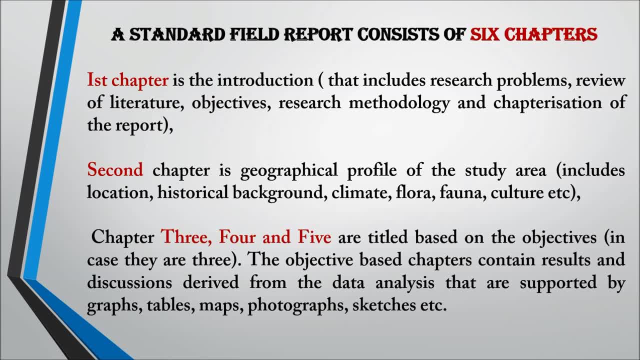 but in a case, three objectives are taken. then third, fourth and fifth chapter would be objective based right, in which it will be supported by all that we have learned: tables, graphs, maps, photographs, sketches, all those things would be included in these three chapters. so these three chapters are going to be the body of your research, right, if you analyze it in a in a way, like a human body. 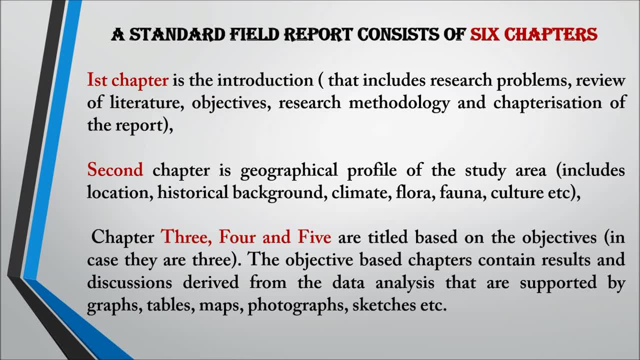 so head of your research is introduction. body of your research is going to be these major three chapters, isn't it? so you remember that in a research, completeness is dependent upon your objectives, so the objective based chapters would be the most important body part. right then chapter 6 is the summary and 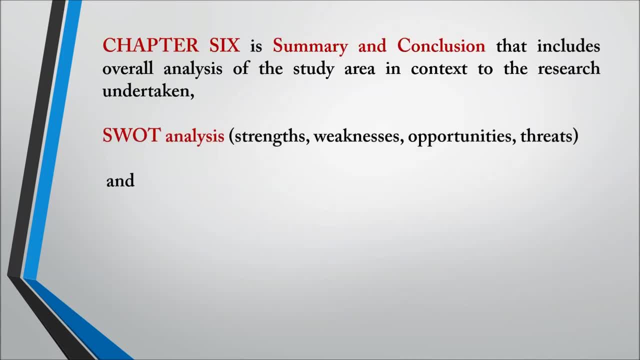 conclusion, which will include swot analysis or many times swoc analysis. so strength, weakness, opportunities, threats or challenges. so SWOT or SOK analysis, because this has to be an assessment, final summary and conclusion part. so you can also provide a summary and conclusion part. you can also provide a sort analysis, maybe other kinds of such analysis, like economic analysis. 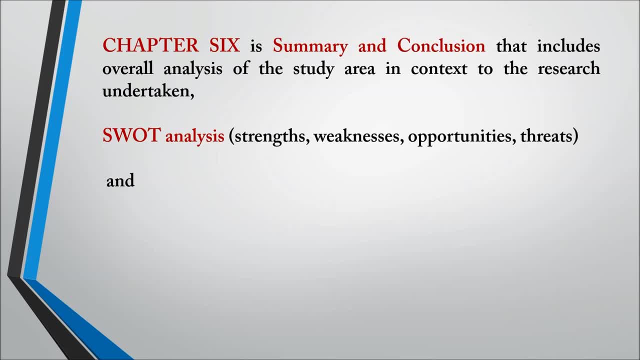 so cost benefit analysis, certain analysis you can put in the last summary and conclusion part. right and recommendations are the most important point that we also discussed in the previous session, because the map of recommendation, the map of intervention, area of intervention, these things have to be coming in the last summary and conclusion chapter. so recommendations: 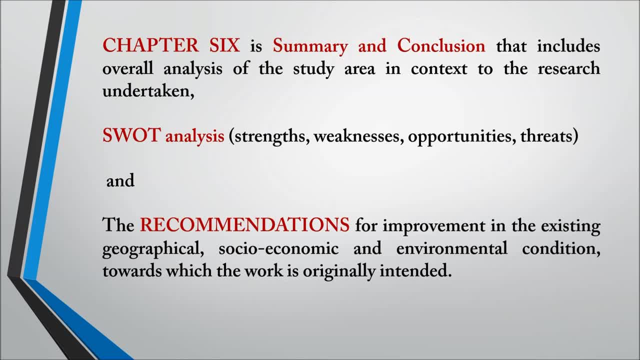 are important because a researcher has gone to the field, sought information, analyzed it, and now he, she, is capable enough to recommend something for the improvement in the area geographical, socio-economic, environmental, without any condition. but a recommendation part is must, isn't it? so whatever recommendation, but remember, recommendations should not be general, it should be specific to the 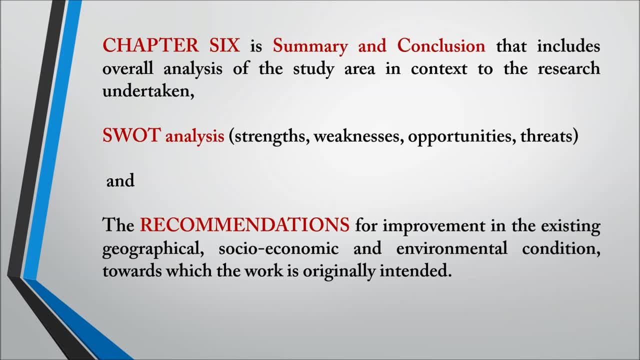 area you're talking. suppose if you have studied climate change impact on agriculture in a particular district of india, you have studied climate change impact on agriculture in a particular district of india and you are talking about general climate change recommendation, then that is no way admissible in this kind of research. so it has to have impact on the context. so recommendations: 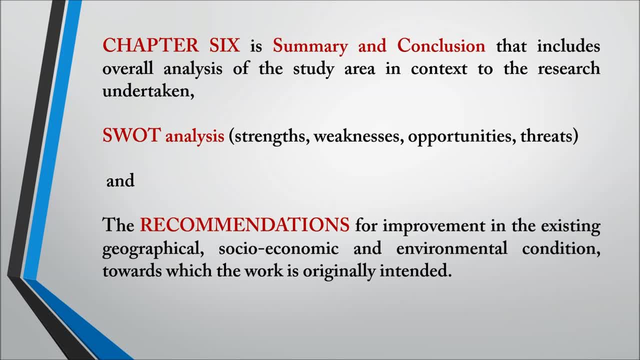 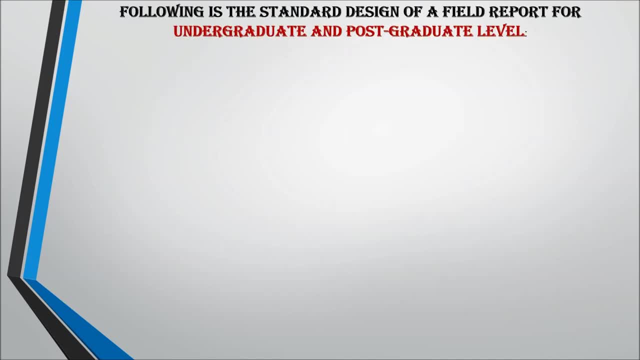 should be always context basis, never put any general recommendation, isn't it? now? what is the standard design? today, we are going to finalize the standard design for undergraduate and postgraduate level. it can not be the standard design. it can not be the standard design. it can not be the standard. 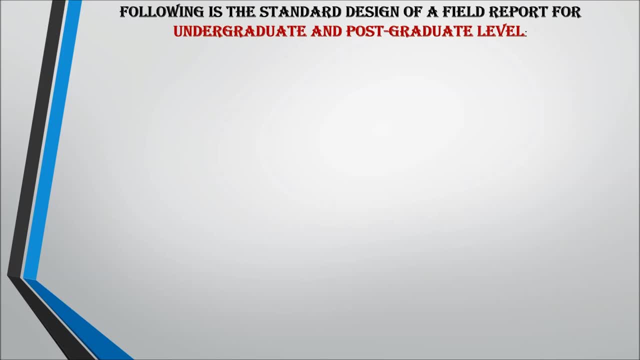 it can have little bit variation as well in depending upon your research and context of study, but i'll only tell you the undergraduate and postgraduate level of a standard design of field report. okay, so let's begin. first page is title page, in which you are mentioning your entire title. 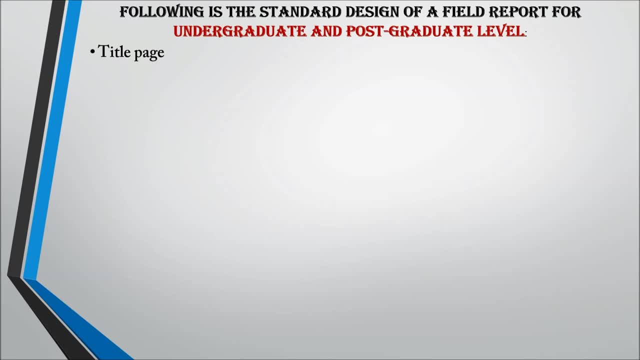 your university name, your roll number, maybe about yourself, your supervisor's name. so this is going to be the title page, right. then we have certificate, so it includes researchers as well as supervisors. so second is your certificate page. then you have your acknowledgement page, where you are acknowledging all the people involved directly or indirectly and all the institutions involved. 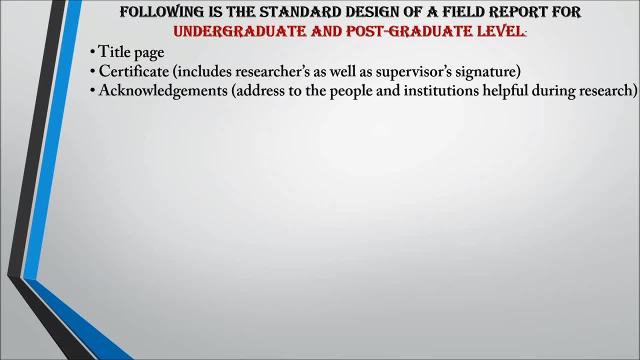 directly or indirectly, whose help you have sought while making the research. so do acknowledge. don't just write acknowledgement for the sake of writing acknowledgements. it has to have proper means to address all those people and institutions who were helpful to you during your research. right that's. 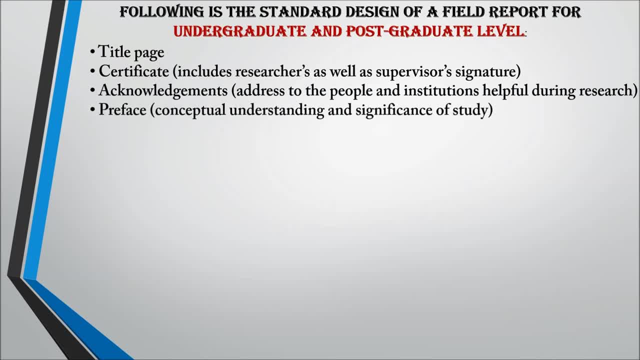 why acknowledgement matters, preface- now it is the preface. it means it's kind of an introduction to what you have done in your study. so it is the conceptual understanding and your significance of your study. this is what you are going to put in your preface. so concept of your study and significance of your study. why? 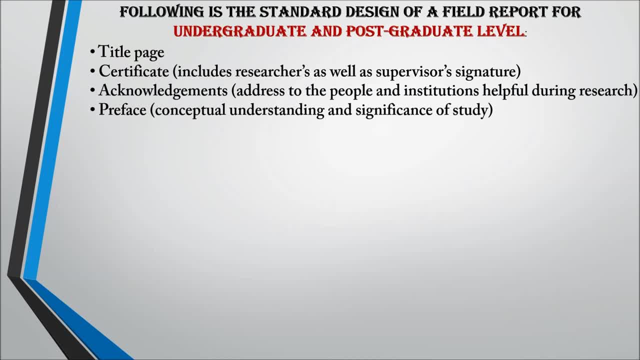 have you done it? what is the need for it? this is what preface is all about. all right, then contents. so you have to design your content page that includes all the components with page numbers. remember, put page numbers mandatorily in your components of the content right and make it in a same format. don't use 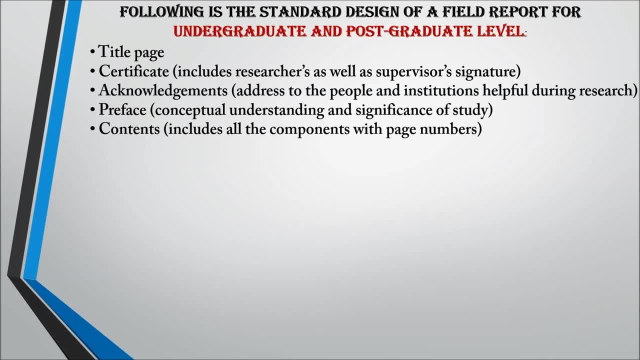 somewhere capital, somewhere small, so make it a uniformity in the content section. then list of figures, that is, graphical representations, have to be put in a separate list of figures used in the entire chapters if you have six chapters. so how many figures were used? 30 figures, 40 figures, so 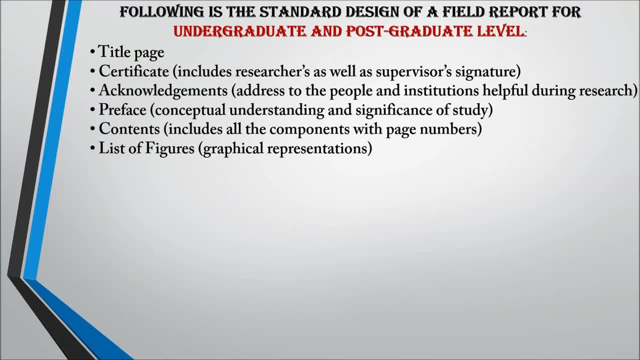 make a list of figures with their titles and page numbers. similarly, for the list of tables, tabulated statistical analysis, with their page numbers. list of plates, that is, maps and photographs. all right, so list of figures, tables, plates. that is the next sequence. then come to the first chapter, that is, 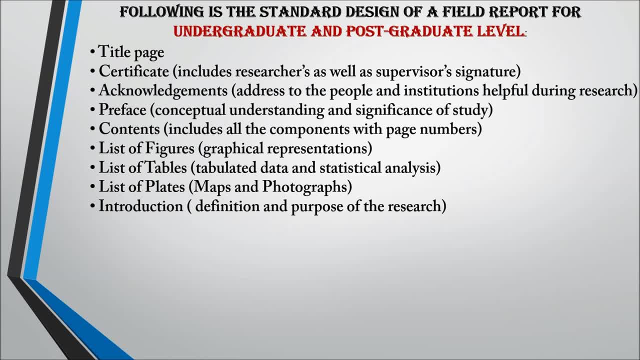 your introduction part. so definition and purpose of research have to be written. review of literature is review of previous research already there conducted. so that is what you have done, you have to review it, don't just write it. what you have done, you have to review it. reviewing itself is: 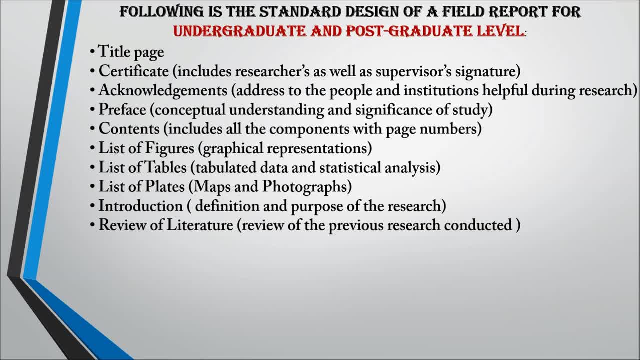 a different kinds of study. you have to train yourself how to review a literature, so write it. so basically, go and study the rubric, don't simply write. oh, this is my comment. don't simply compare the학ive right, because you want to look at the feedback. MY 2230, in which 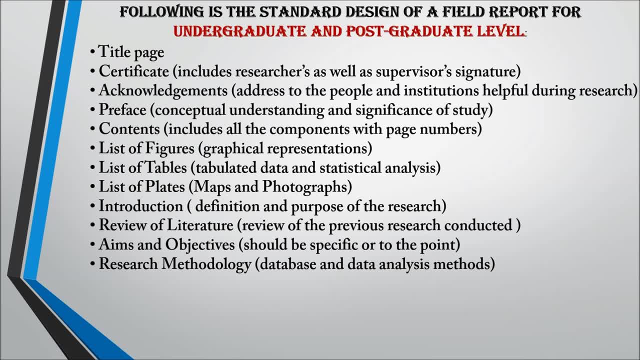 there is no for find works. it is the Window of time. now let's get out of here. yeah, i have completed my test and you can write an end of and need the final review format. then aims and objectives should be clearly specified. then research methodology: again we talked in the last session- the database. 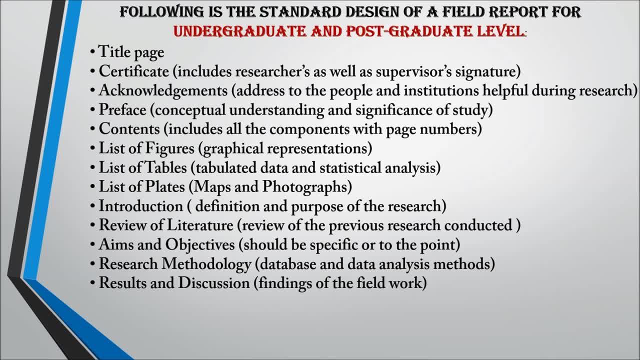 and data analysis are two segments of research methodology. it needs to be clearly shown specifically. you can show it through a floor diagram right then results and discussions, that is, the findings of the field work that you have done, and then, finally, summary and conclusion. many times this is a question that what should be put at the end: references or selected bibliography. 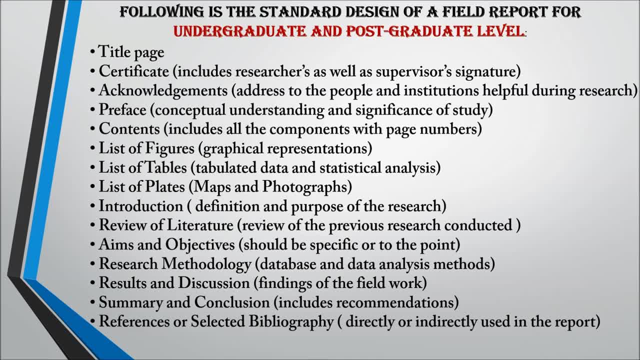 see references is which you directly quote in your search. but many a times there are certain references that you have not quoted directly but you must have read it for your conceptual understanding. so selected bibliography is what were the selected texts that you studied for the research work so directly or indirectly combined together? it's bibliography, directly only it's. 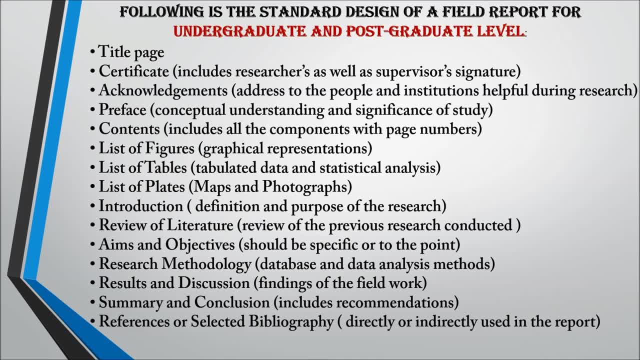 references so many a times. your mentor or supervisor may ask you to write separate references at the end of each chapter and then finally write a selected bibliography at the end so you can change it accordingly. but this is the largest standard framework design of a field report. so remember the design from title page to the selected bibliography and the last part will. 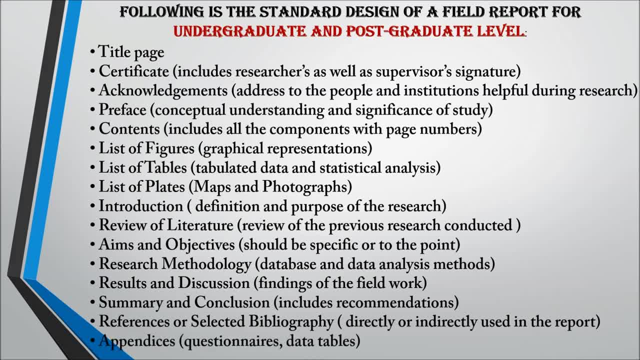 contain the appendices, that is, questionnaires and data tables that you use during your field report. so your field survey, so you can put it in a blank format unfilled, your databases and your questionnaires that you have utilized for your analysis. so this is the complete design of a 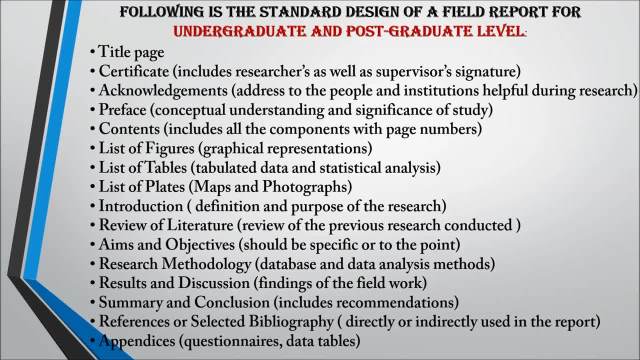 standard report at undergraduate or postgraduate level. any variation would depend upon your context, your mentor and your institution. if your institution or your mentor has a different framework, then you can change it. but this is a standard design of a field report. then these five elements matter, because Mage� and Read are based on field survey. all right that. 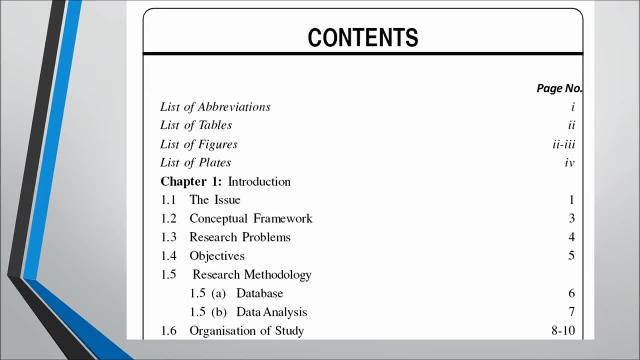 we do in geographical studies and many other social science research as well. now illustrations: so that is contents that i was talking about. so you have to make a content page. so your content page design may look like this, something like this: so list of abbreviations, list of tables, figures, plates that you can write in again, page numbers, then you can write your. 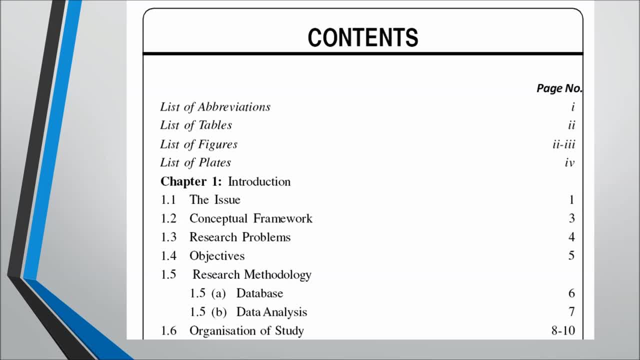 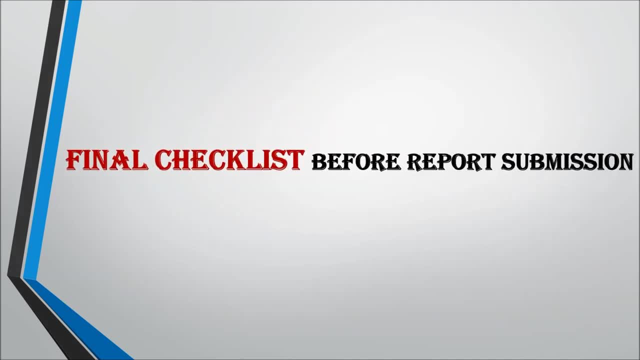 chapter one, introduction. and what are the components? again, 1.1, 1.2, 1.3. that right, so final checklist before report submission. so what is the final checklist? finally, before submission, remember that you need to understand that you need to provide a final checklist for yourself, remember, print. 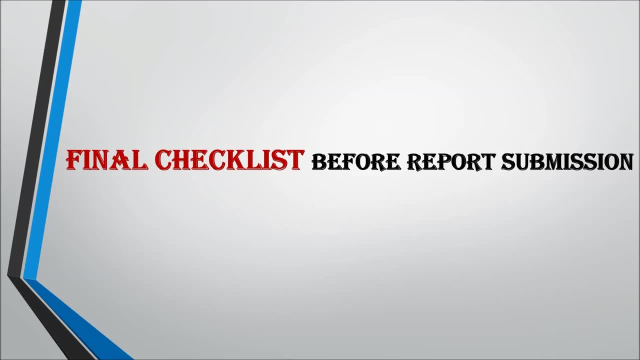 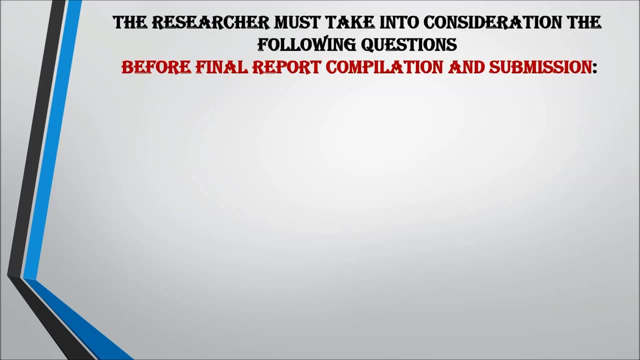 this checklist and put it on your desk. and finally, the day of submission. before the day of submission: just take a pen and tick mark, okay, so put a tick against this checklist. that have you done that? so what are the questions involved? let's look at the compilation of the entire submission of final report, in which a: 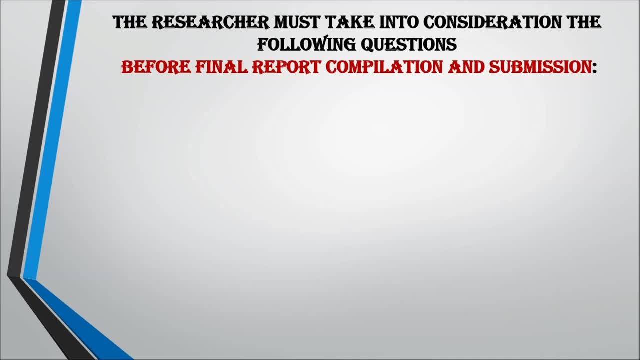 researcher must address all the questions. so what are the questions? first question: have all the references been quoted at the end of statement of paragraph with author's name? and here this is the first thing that you need to check after you have completed your report. have you quoted all the? 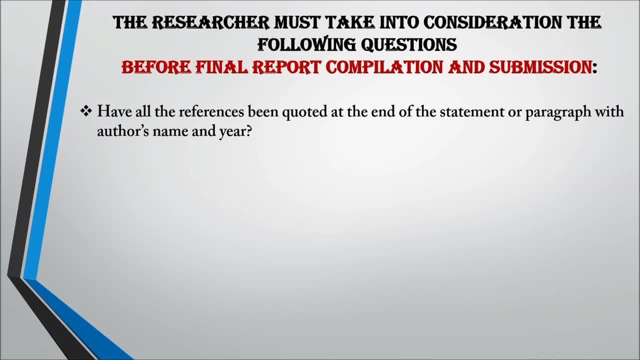 references at the end of statement of paragraph. have you quoted all the references at the end of statement of paragraph, author's name and year? if you have taken it from some reference, you must quote it, okay, otherwise it is a plagiarism. then is full reference being listed at the end in the stated reference section. 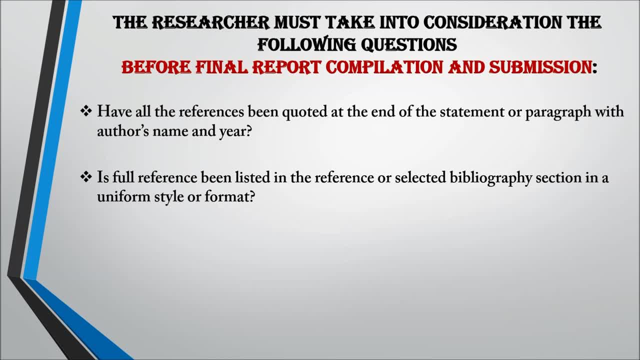 or selected bibliography section in a particular format that you decide. then have all the diagrams, graphs, maps, photograph, sketches been clearly labeled? so labeling all these aspects- maps, diagrams, graphs, sketches, photographs- is necessary. okay, so you must check that. then again, check that: do all tables, graphs, maps, photograph, sketches have titles and sources, as we discussed. 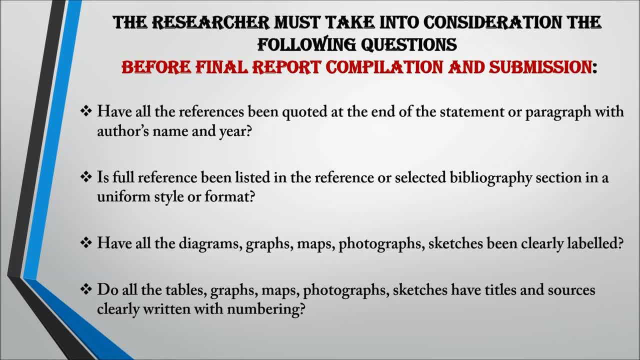 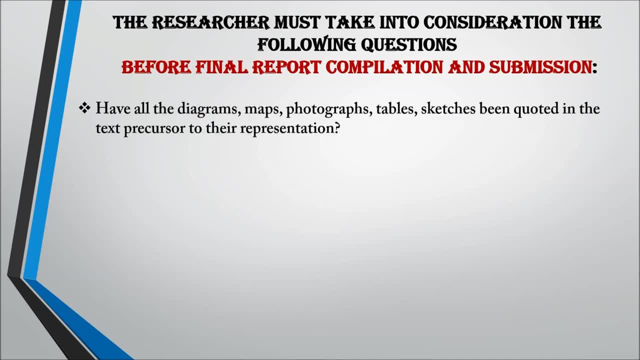 in yesterday's the earlier lecture session. first right, then also check: have all the diagrams, maps, photographs, table sketches been quoted in the text precursor to this representation? this is point where you need to emphasize. you must discuss in your paragraph first and then put your diagrams and maps and photographs. don't put your diagrams, map, photograph first and then. 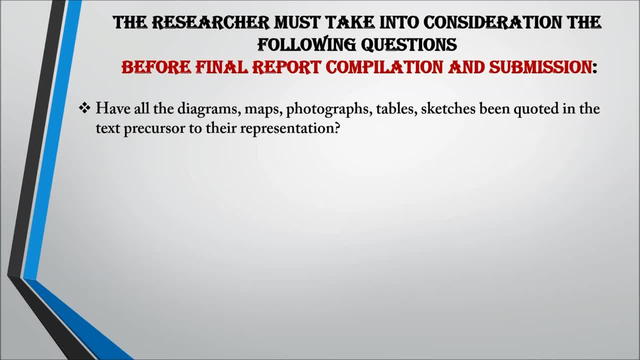 discuss about it. i hope you understand that first you are discussing it and in your discussion you are quoting it. that in the following diagram you can see what i am quoting in the text. that is how a reader would understand. so first talk about the diagram. map graphs. 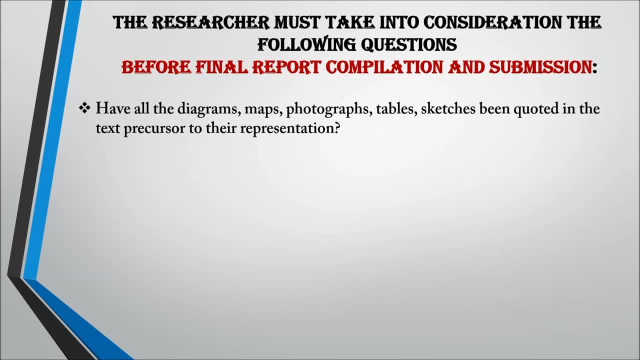 and interpret it and then, in bracket, you can quote it for the representation and then put the graph. okay, so that is how our report is written. can all the tables, graphs, maps etc. be comprehended by you reader? remember, it should be easy to comprehend. don't make up too much of a complex map or a graph. 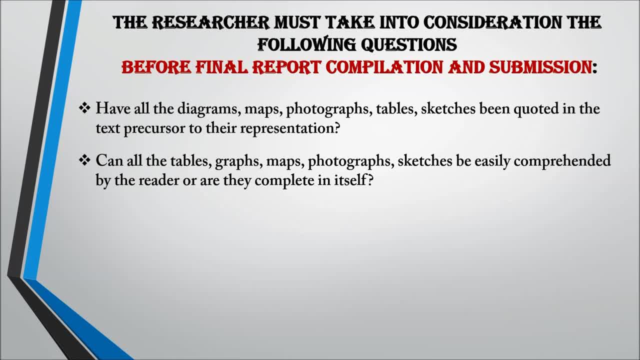 or a sketch. okay, it should be easy to understand for any reader. right have copyright laws being taken into account? this is very much important because if you are using somebody else's material, you must put a reference to it, acknowledgement to it. if you're not using it, then there is a copyright.